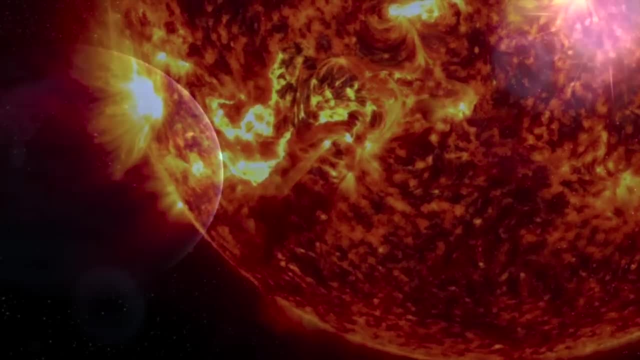 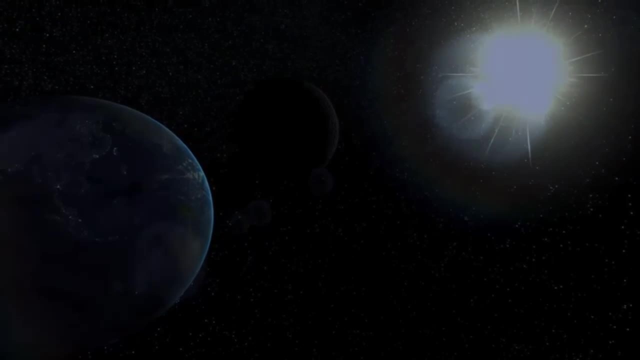 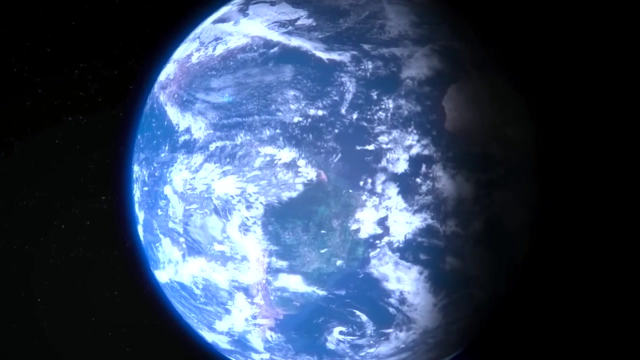 It is not the biggest or the hottest or the oldest. What makes it special is that it is the only known star to support a planet that harbors life Like the Sun. the Earth is not a special planet in any way, Not exceptionally large or small, hot or cold or even composed of unique elements. 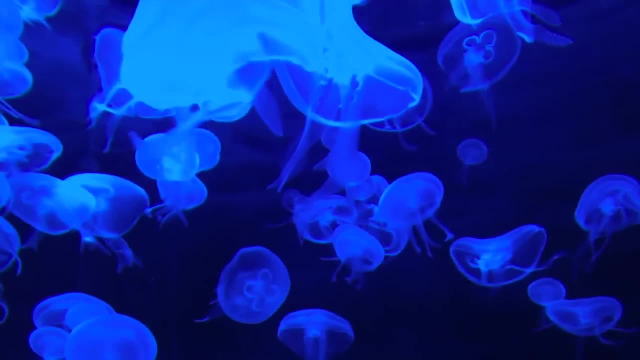 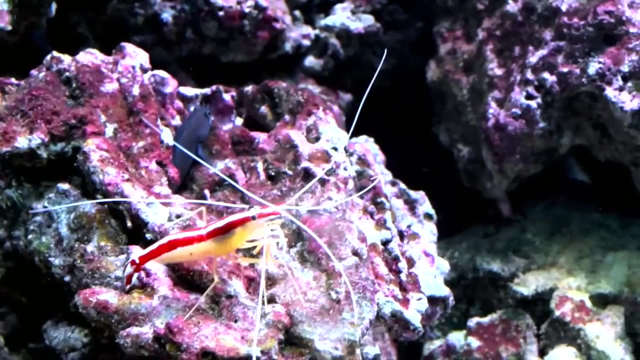 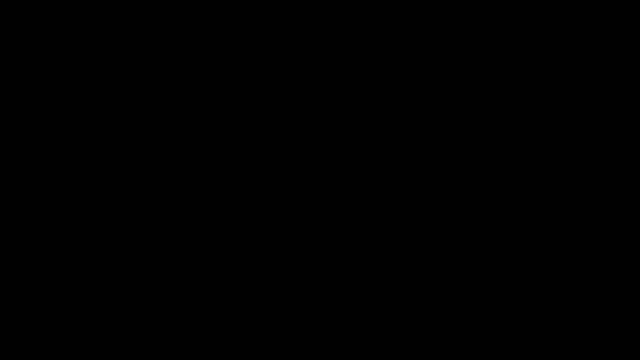 But it is very special in that it is home to life. Nearly 9 million unique species of living things roam our planet, something that we have not yet discovered anywhere else in the entire universe. The study of this exceptional place is a great opportunity for us to explore the universe. 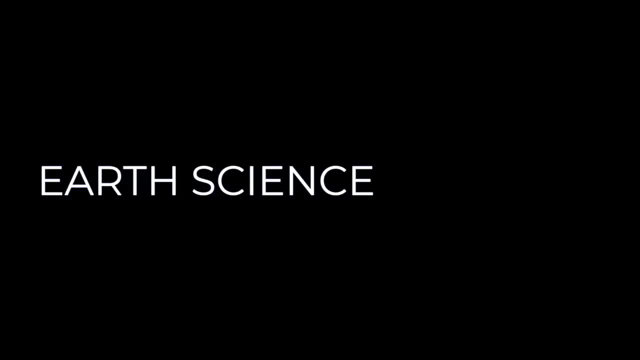 and explore the universe. The Milky Way Galaxy, our local neighborhood in space, is appropriately called Earth Science. This field can be divided into three main areas: Astronomy, Meteorology and Geology. Astronomy is the study of the entire universe, including galaxies, stars, planets and moons. 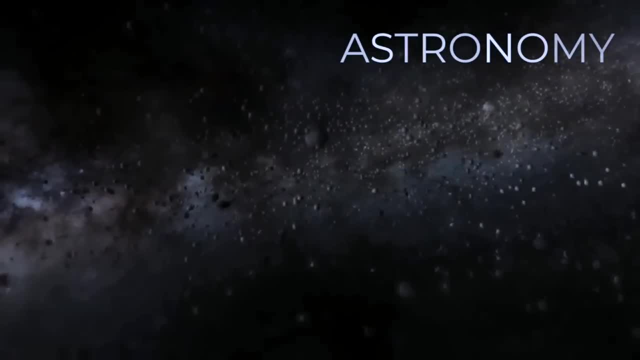 Astronomers explore the laws of motion and gravity and how they control the movement of the Earth and all other celestial objects. Astronomers explore the laws of motion and gravity and how they control the movement of the Earth and all other celestial objects. Astronomers explore the laws of motion and gravity and how they control the movement of the Earth and all other celestial objects. 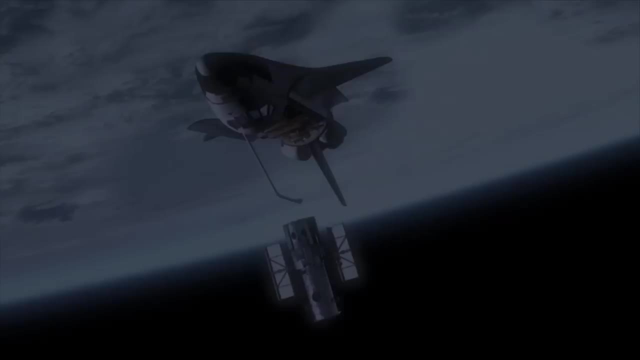 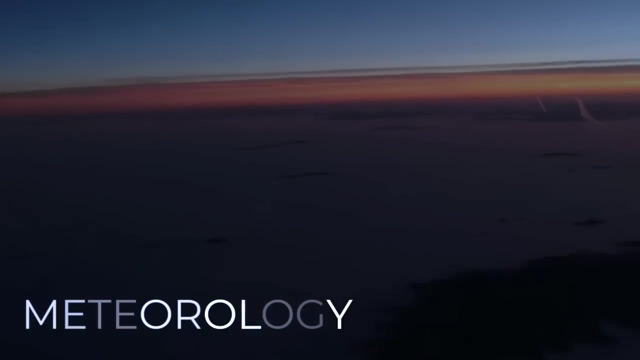 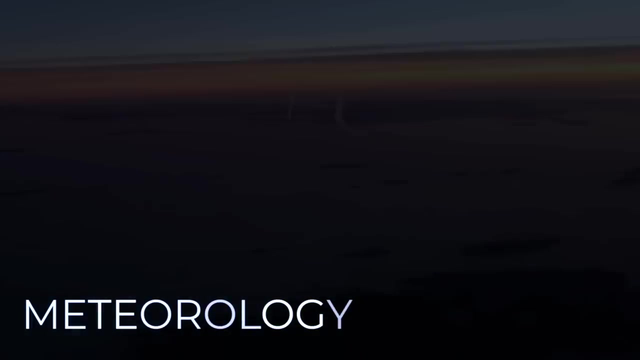 They use massive telescopes to peer back into time to better understand how we got here and where we are going. Meteorology is the study of the Earth's atmosphere, The thin, fragile shell of gases surrounding our planet. Meteorologists explore everything from weather and climate patterns to global climate change. 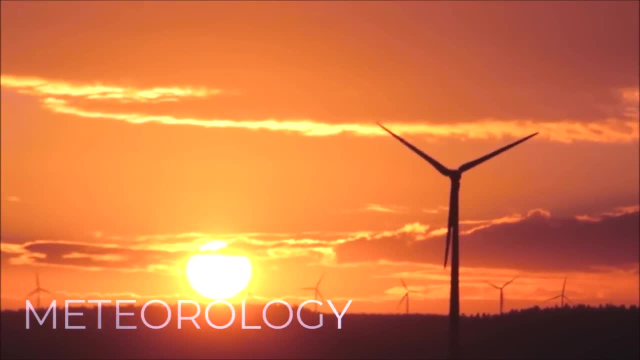 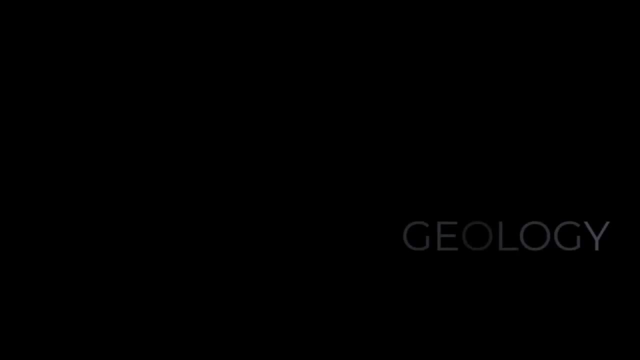 They strive to understand how energy travels and is transformed through shot–ins. OKAY, WE'RE BACK TO ART. YOU ARE MADE formed through the air and water surrounding the earth. Finally, there is geology. Geologists study the solid earth and how it changes from the surface. 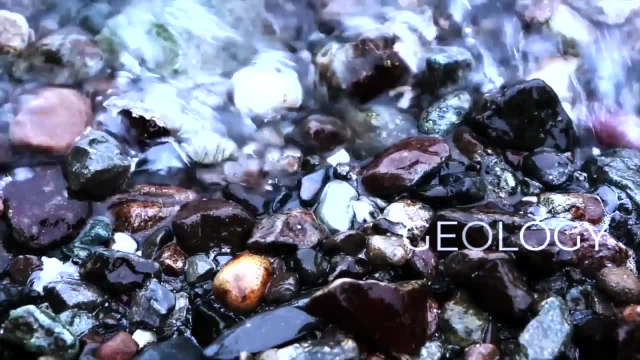 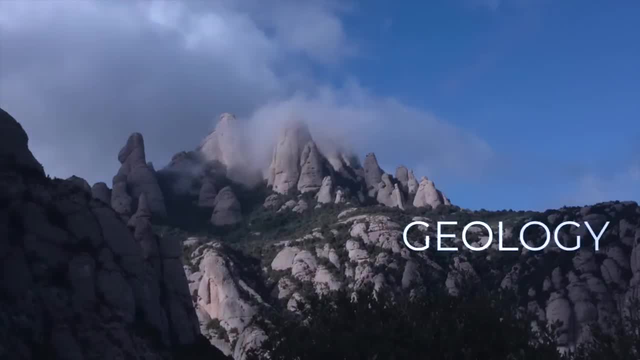 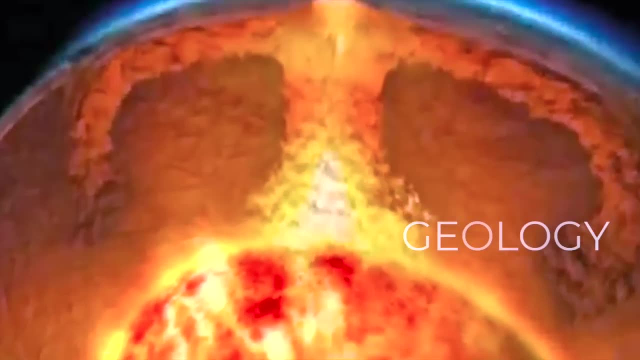 down to the core. They examine rocks and minerals, volcanoes and earthquakes, the oceans and various landforms and landscapes. They also hypothesize about the characteristics and conditions of the interior of the planet. down to our iron-rich, dense hot core Earth, scientists strive to understand the